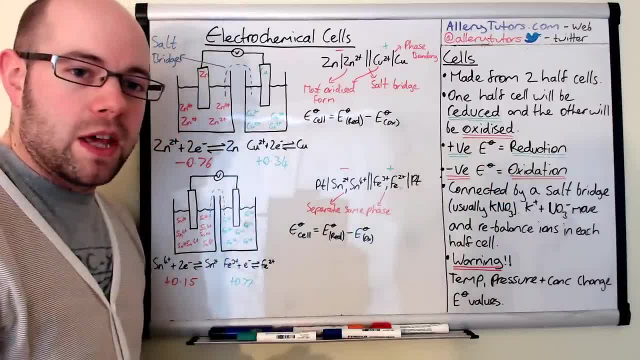 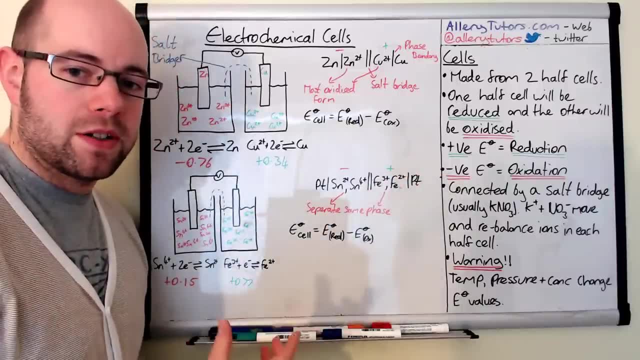 positive E0 values will mean that the reaction is more likely to be reduced, and negative E0 values will show that the reaction is more likely to be oxidized, and we're going to use that quite a lot. throughout these examples here I'm going to show you where we can apply them. They become: 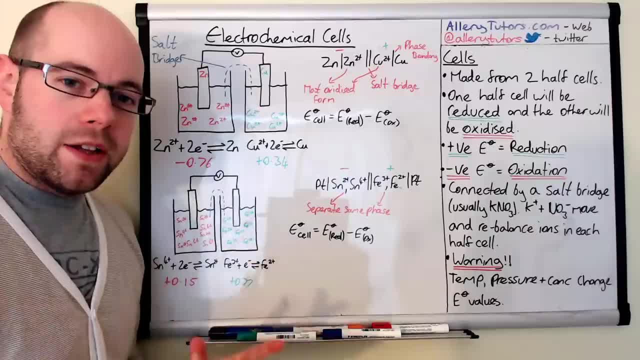 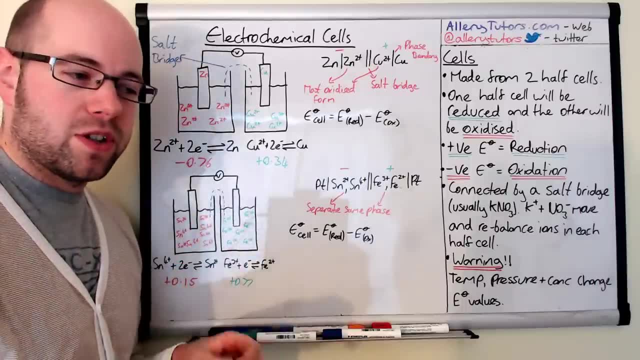 particularly useful when you're working on the E0 of a cell. Full cells are connected by salt bridges, and this is the blue dotted lines that you're seeing here. The salt bridges are basically just bits of filter paper that's dipped into a very saturated 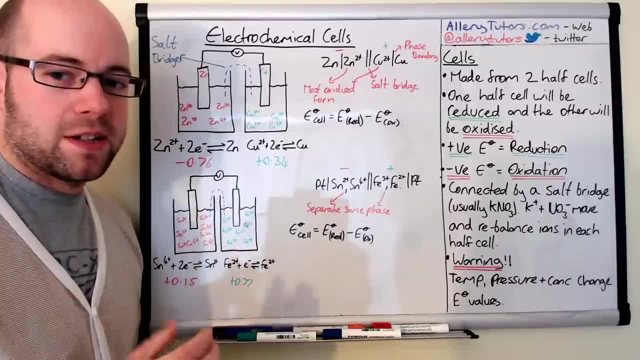 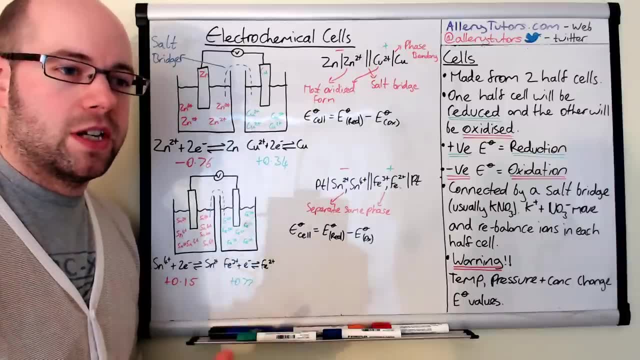 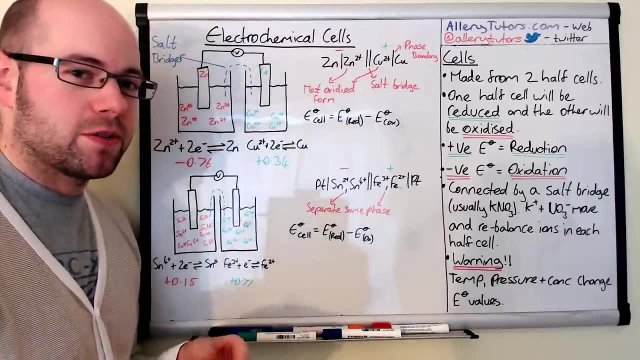 salt solution. Now, normally the salt of choice is potassium nitrate really, really soluble and can move easily across the filter paper that we've dipped in. So it is really important that we do this, and its main purpose is to readdress ion balance in the two half cells. 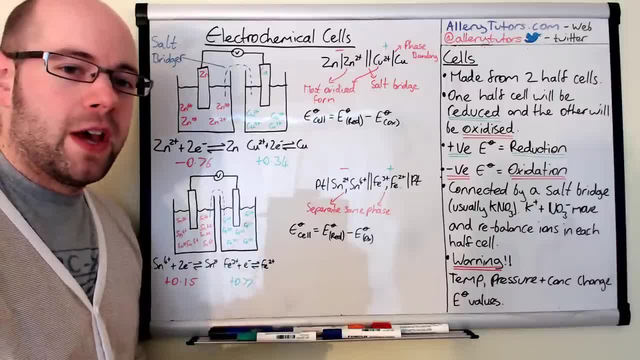 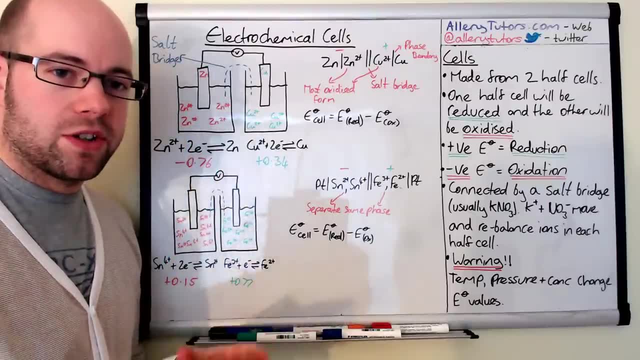 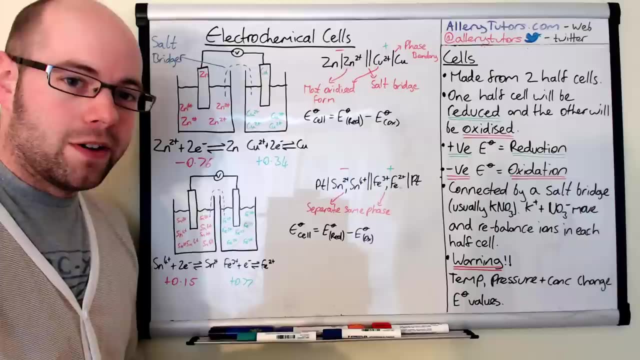 as well. So that's about as much as you need to know for the salt bridge. You've got to be careful, though, that any values that we're using here are assuming that we have standard conditions. That means we have 298 Kelvin, 100 kilopascals of pressure, and also that the concentrations 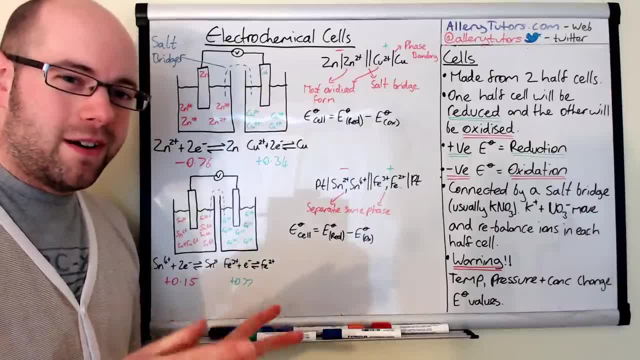 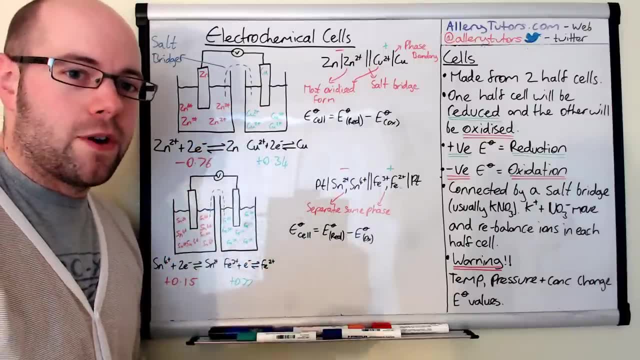 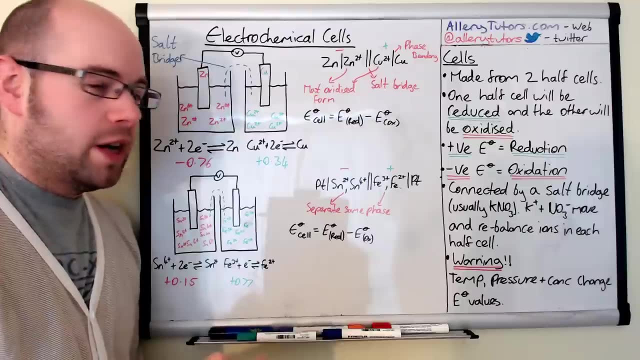 of any solution used are one moles per dm cubed And obviously it's very difficult to get the exact values and you'll find that when you do these practically, that your values will differ from what it says in theory. So you have got to be careful about that as well, and there will be another video in. 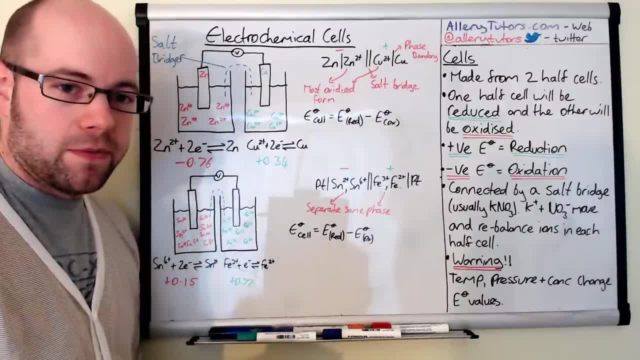 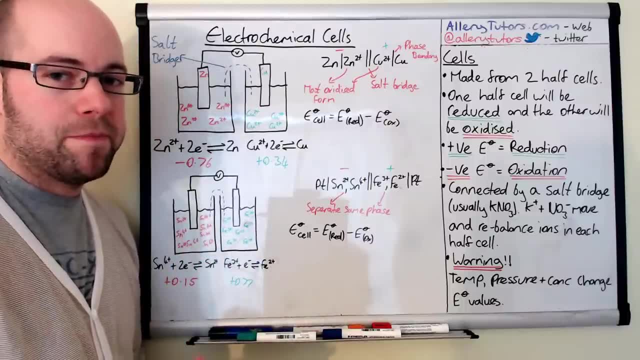 this playlist that looks into the effects of concentration and temperature on these reactions as well. but I'm just going to go through the basic electrochemical cells for the time being. So I'm going to go through two examples and I'm going to show you how we do the cell representation. 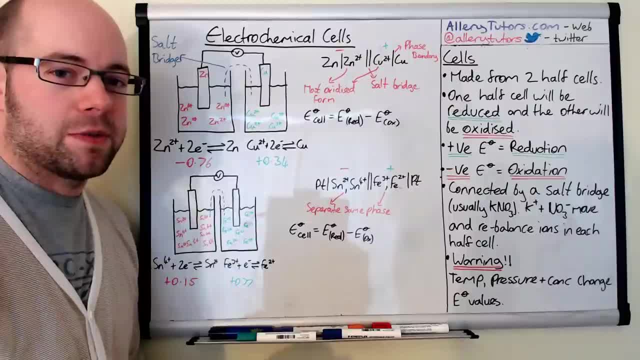 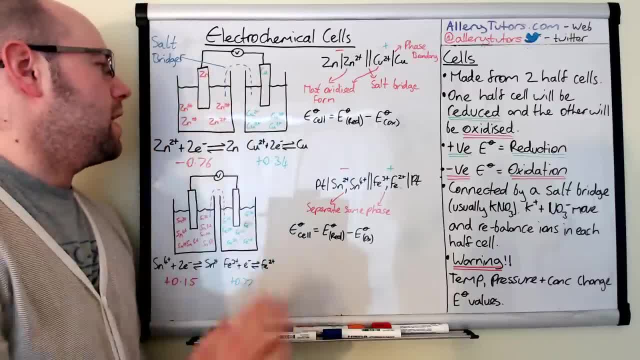 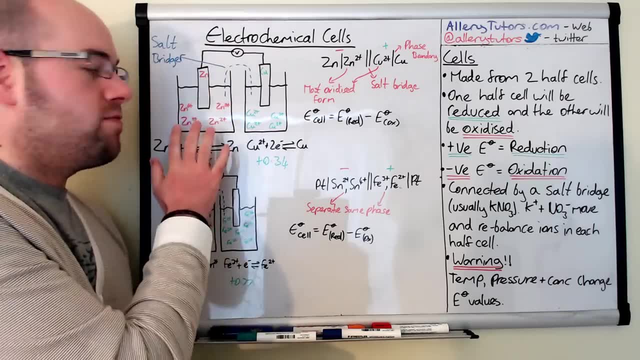 This is a full electrochemical cell And we've decided to link the zinc half cell with a copper half cell. So you can see here that I've done. anything that's been oxidised, I've written in red, and anything that's been reduced, I've written in green. 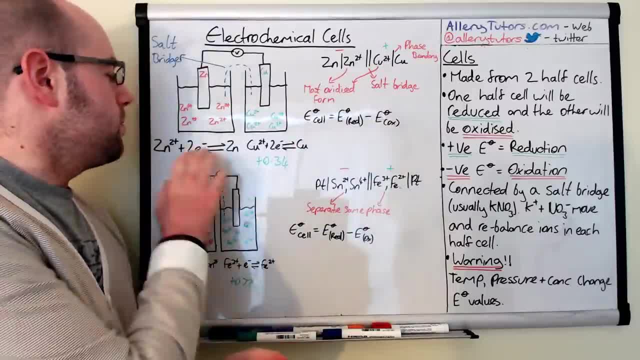 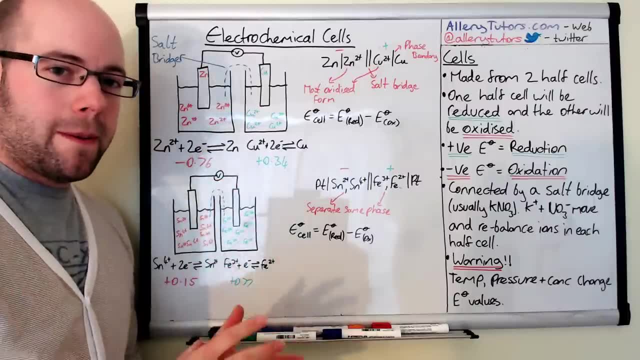 So I've colour coded the whole thing so you can see it a little bit clearly. So I've started with this one here. This is zinc. Now you'll notice that all of our equations here are written in the reduced form. What that means is that your electrons are written on the left hand side, irrespective. 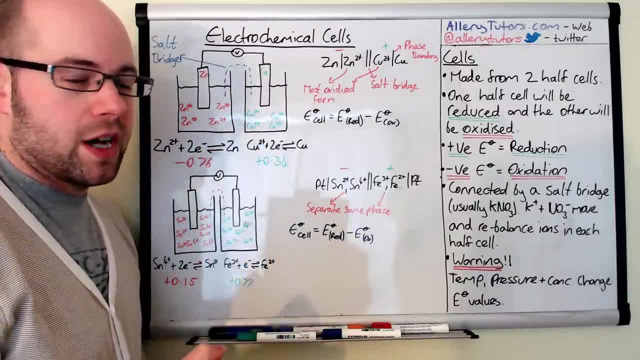 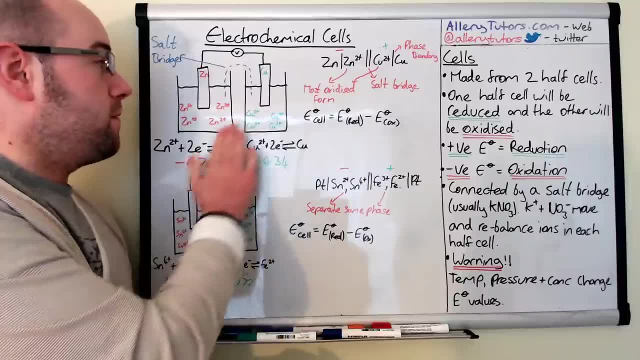 whether the reaction is actually being reduced or oxidised. We always write them like that. it's just a standard way in which we represent them. So I've written down the equations for the two half cells here. So this one is zinc. two plus two electrons will form zinc, and this one's copper. two plus 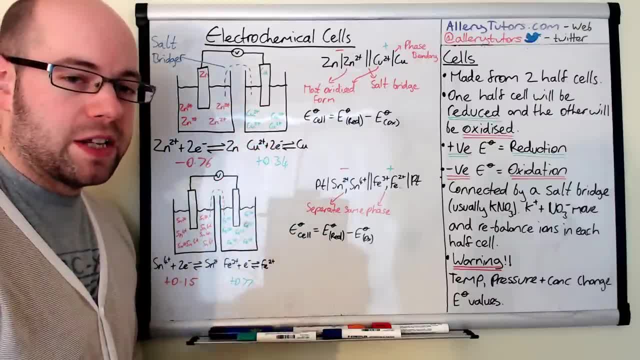 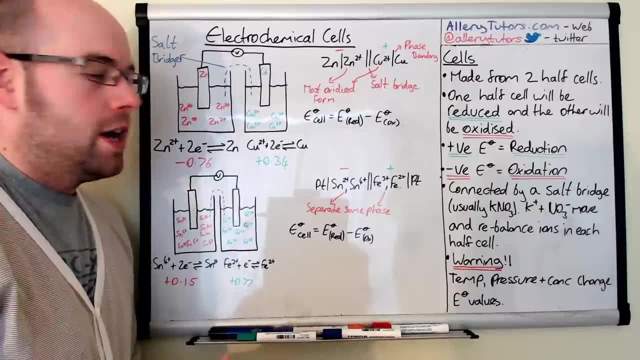 two electrons will form copper And I've written underneath the standard electrode potential for each half cell. Now in the exam you'll be given these. you're not expected to remember these values. So we've got minus, nought. point seven, six here. 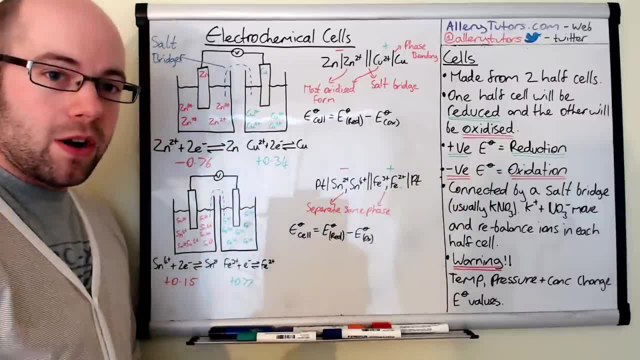 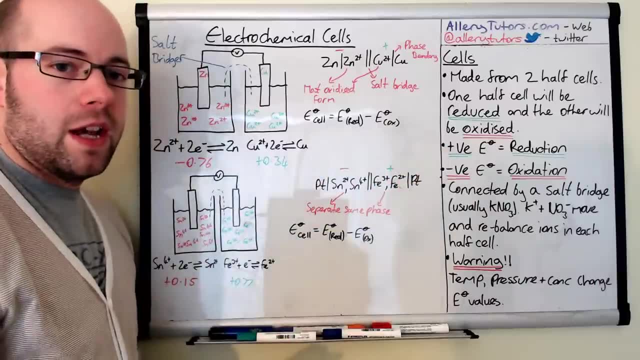 Remember minus E- nought values. That means this is going to be an oxidation process and this one is positive, or plus nought. point three, four, and that tells us that this is a reduction process. So we can see, here we've got zinc and zinc, two plus. 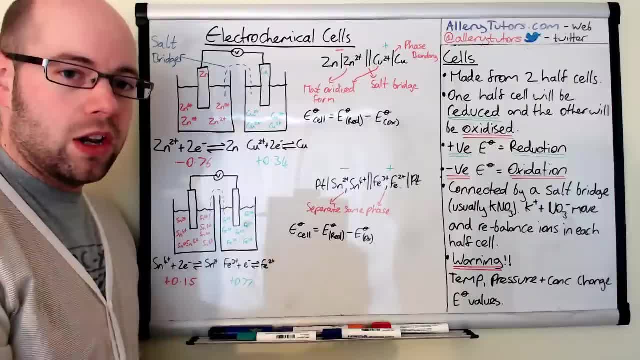 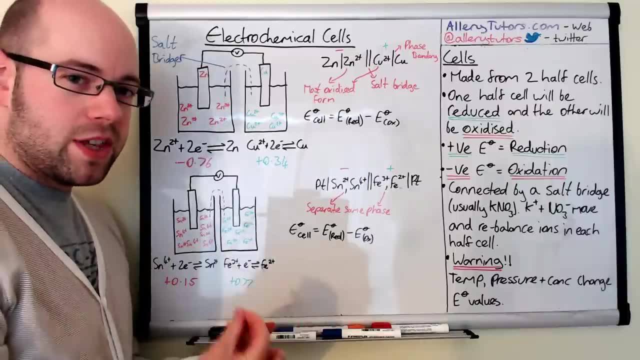 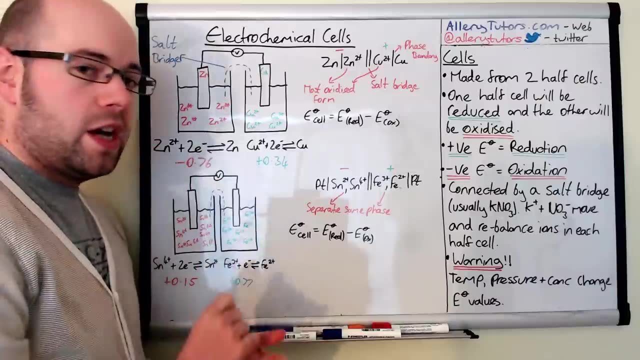 Now because this has been oxidised. oxidation is the loss of electrons. So you can see here that actually this is showing zinc two plus accepting electrons. So actually this reaction is actually going to go backwards And that shows us oxidation. So remember, if the front going forward is reduction, then going back is oxidation. 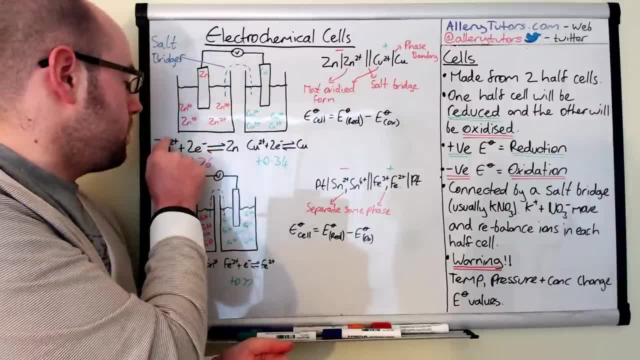 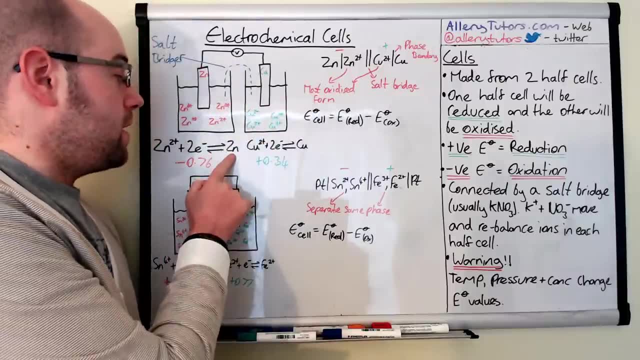 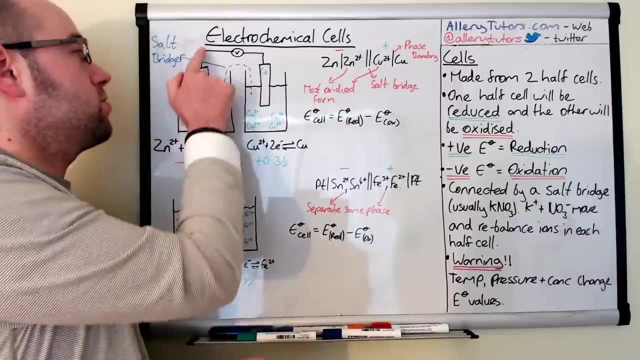 So what's happening here is the zinc is actually giving up two electrons to form zinc, two plus when it's connected with this electrode here. So this is described as oxidation. So the electrons are effectively going to be made by the zinc, and the electrons are 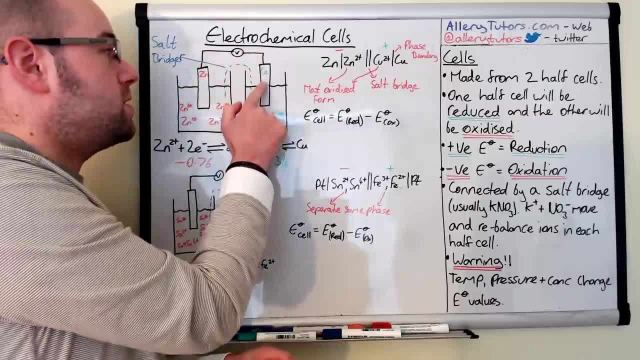 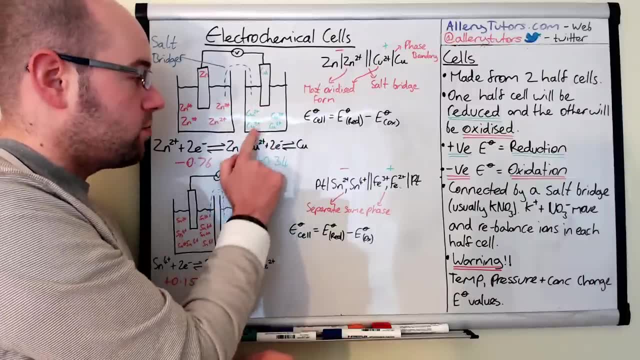 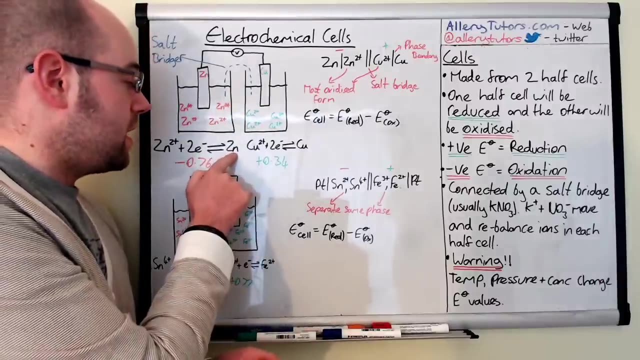 going to go through this wire here, through the voltmeter and down into the copper, and this is going to pick up the two electrons And the copper- two plus in this solution- are going to react to form copper metal. Now what you would observe in this case is because the zinc is going to form zinc two. 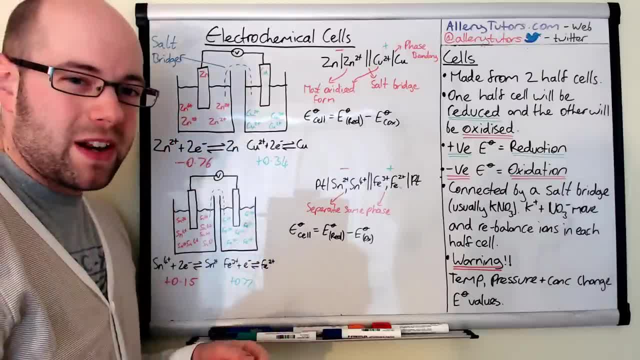 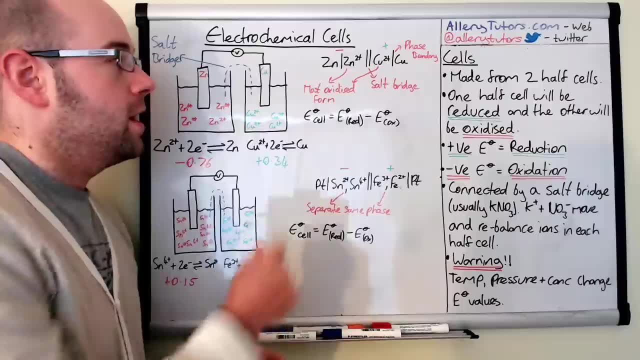 plus, because this is showing oxidation. then the zinc will effectively start to dissolve. You'll get this to start to thin, because obviously a lot of it is being used to make zinc. two plus And on the other side you'll get a buildup of copper around this electrode because the 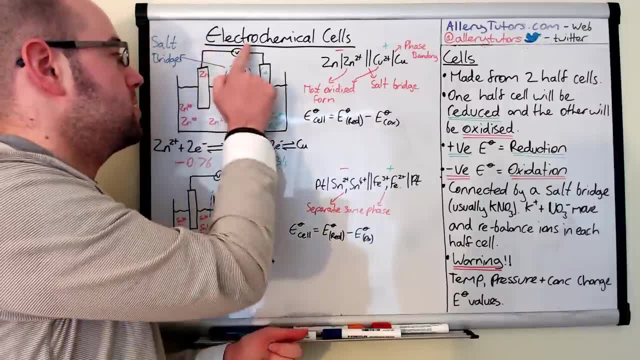 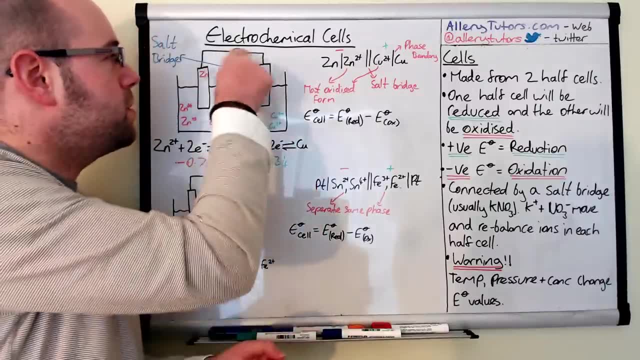 copper, two plus ions are accepting the two electrons And that we're released from the zinc to form copper. So you'll see a thickening of this electrode here and that's what you should observe. And you see, we've got our salt bridge in the middle. 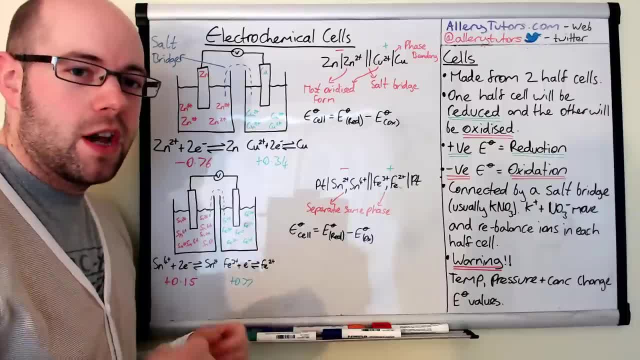 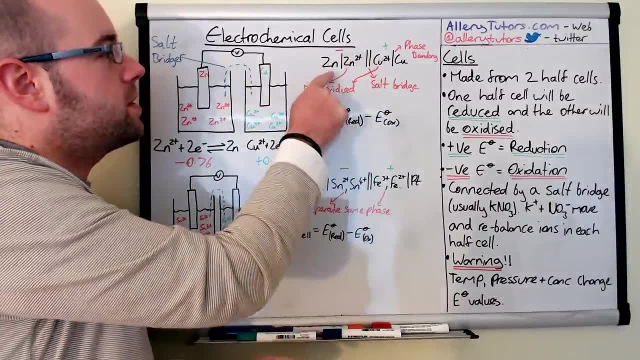 Now we can represent this instead of drawing out beakers and electrodes. we could represent this in a bit of a neater way, in a quicker way. We call this a cell representation here, So you can see here that I've written down our most negative electrode, which in this 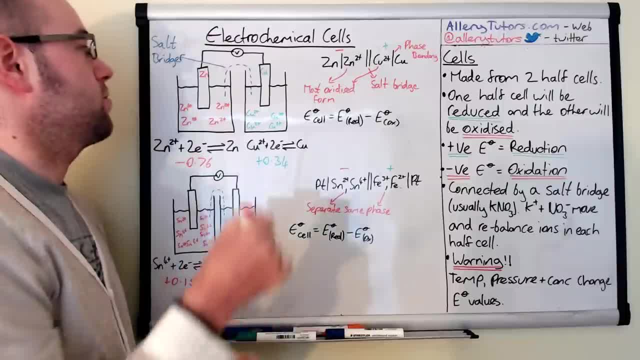 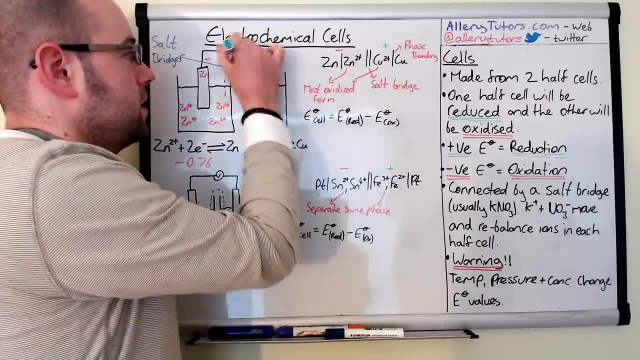 case would be zinc, because this is what's making the electron. So this is going to be our negative electrode And obviously the other side is going to be positive. I'll put that on that side because that's accepting the electrons. So what we do is we write the most negative, the negative electrode, on the left hand side. 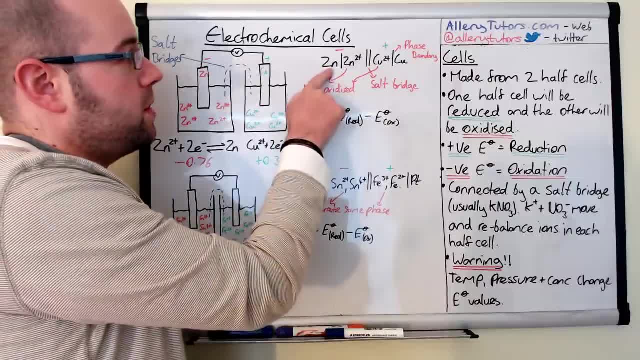 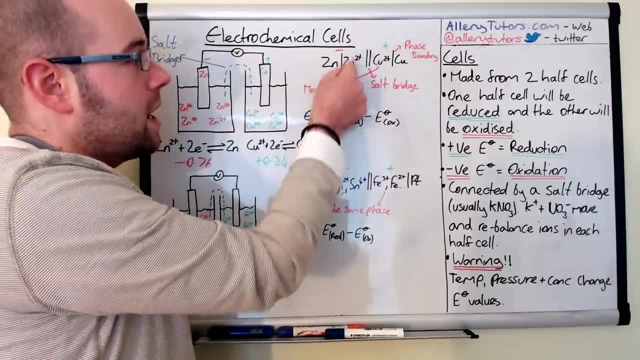 and the positive electrode on the right. Now, what we've done is we represented by writing our electrode, which is the solid electrode, which is zinc. on the left, We draw a line and this line shows the phase boundary. Now, this is the boundary between a metal and a solution. 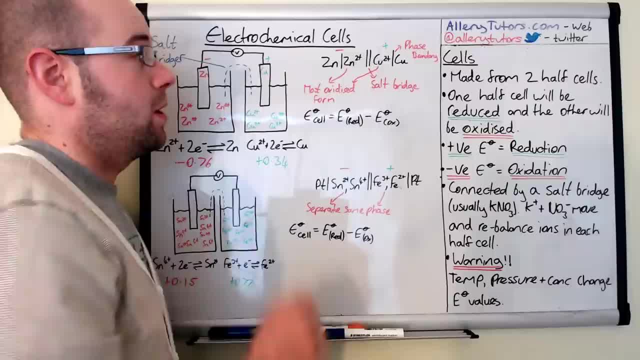 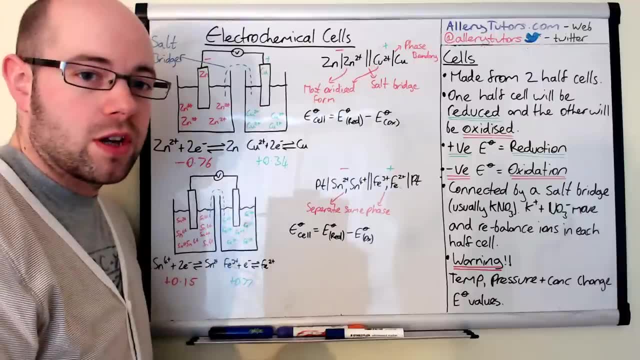 So we draw a line there And then we write zinc two plus closest to the double line which is the salt bridge, And we always write the most oxidized form closest to the salt bridge. So out of zinc and zinc two plus, zinc two plus is the most oxidized form. 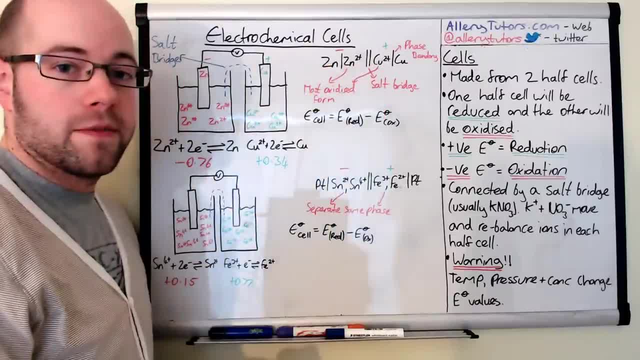 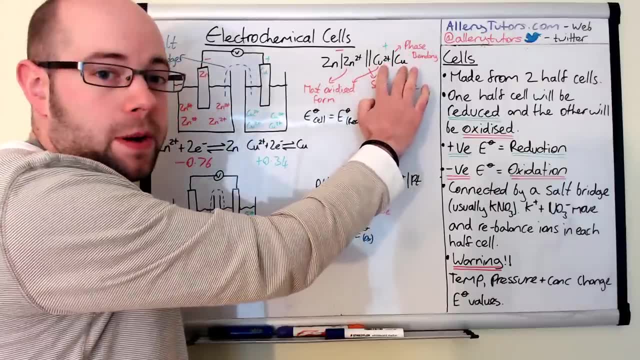 It's got an oxidation state of plus two. This has got an oxidation state of zero. Okay, So if we look on the right hand side, which is the copper electrode, you can see here the most oxidized form out of copper and copper two plus is copper two plus because it's got 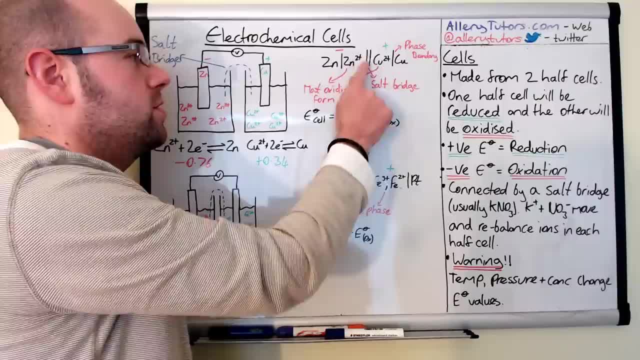 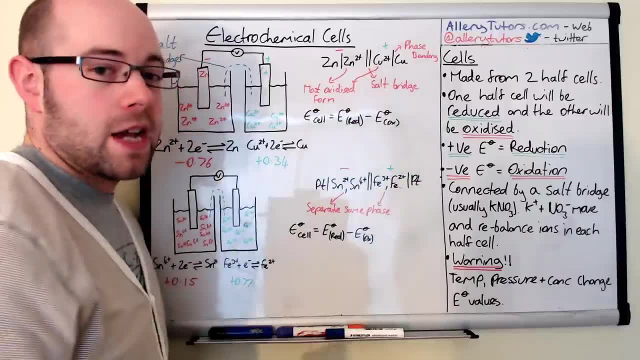 an oxidation state of plus two. So we draw that closest to the salt bridge, as you can see here. And then the lines, just the phase boundary, because we've got an aqueous solution and a metal electrode. So that's how we work that out there. 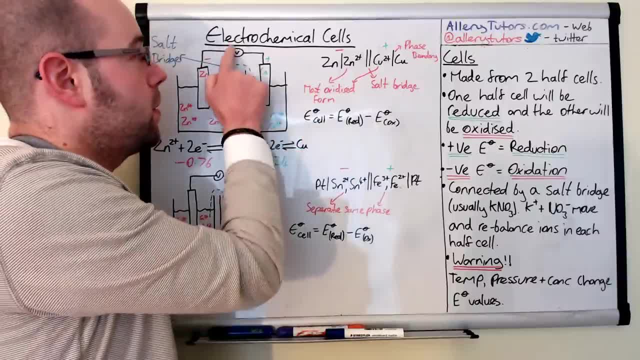 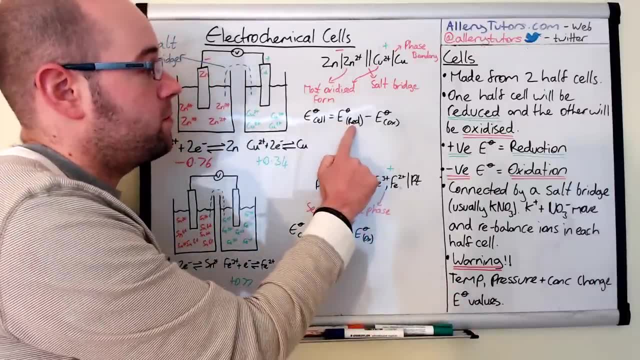 Now we can work out the E naught of the cell and this is effectively what this voltmeter is reading here. This is the potential difference across this, And we can do that really easily by doing E naught of the reduced form minus E naught. 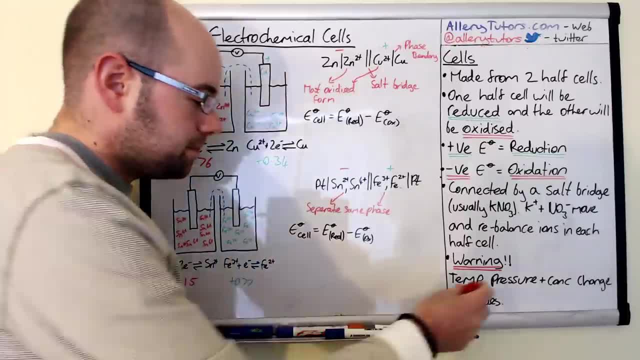 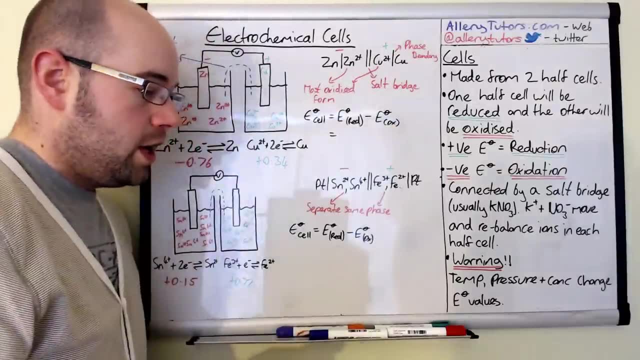 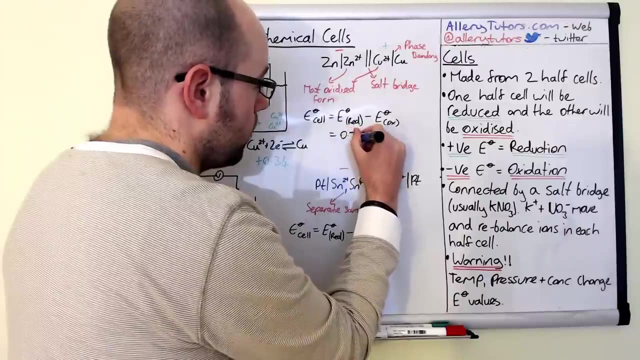 of the oxidized version, Or We can put the numbers in and then we can get our value. So E naught of the reduced form is going to be this one here. This is the copper that's being reduced. So I'm going to put naught, point three, four, and we're going to subtract that away. the 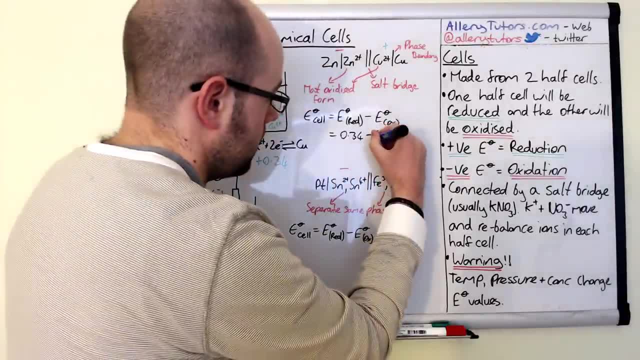 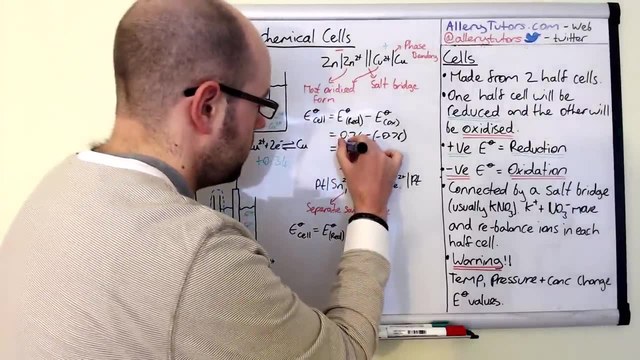 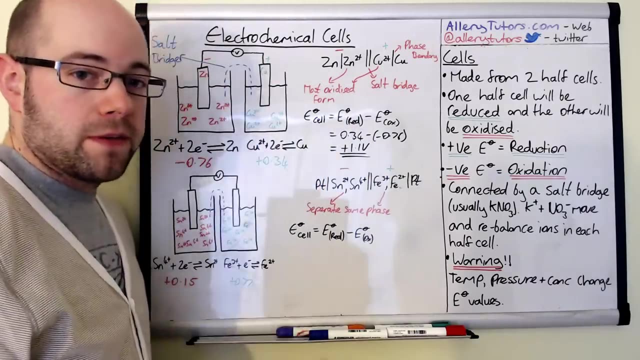 oxidized form. This is minus naught point seven six. So minus naught point seven six, And if we put that in our calculator we should get the voltage or potential difference of plus one point one volts, And that is basically the electron potential of this full cell here. 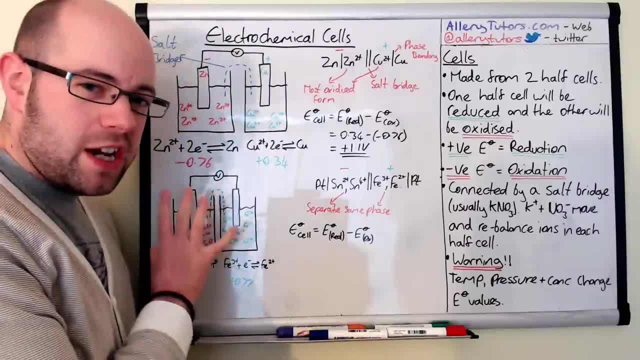 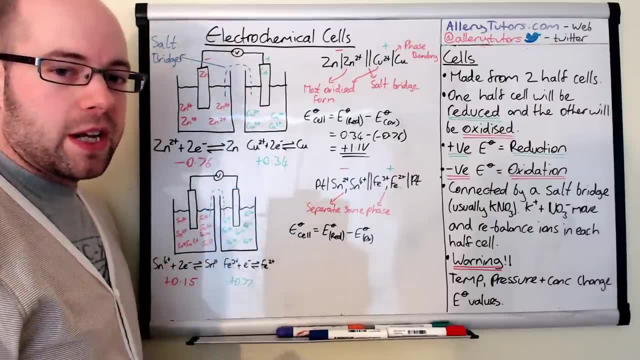 Now I've got another example just below, and I've changed it a little bit, because actually, with this one it's not too bad, because we've got a negative electrode and a positive electrode. Sometimes, though, we can have two positive electrodes and one of them is more negative. 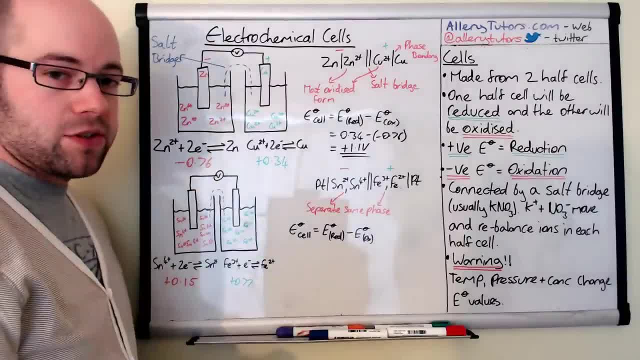 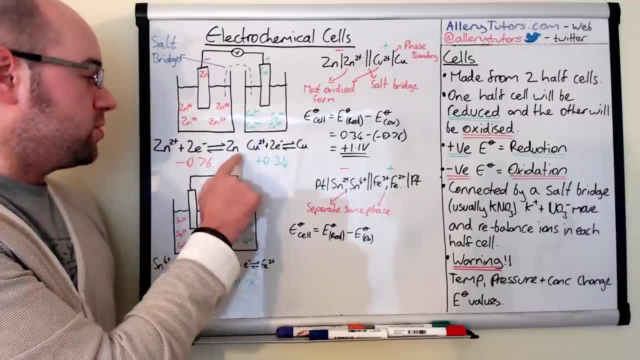 and that would take up the role of the negative electrode. So, for example, I've got this here. now again, I've changed it again as well, because instead of having a solid electrode And it's ion, we've effectively got two solutions here. 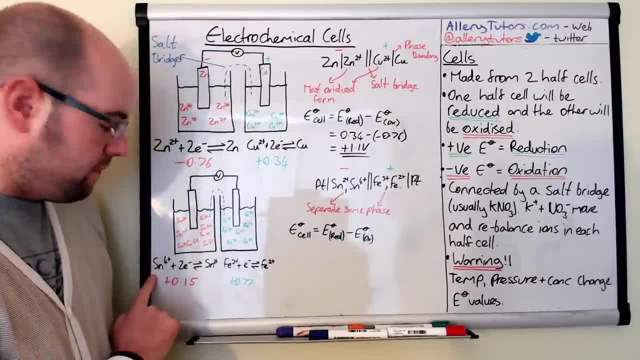 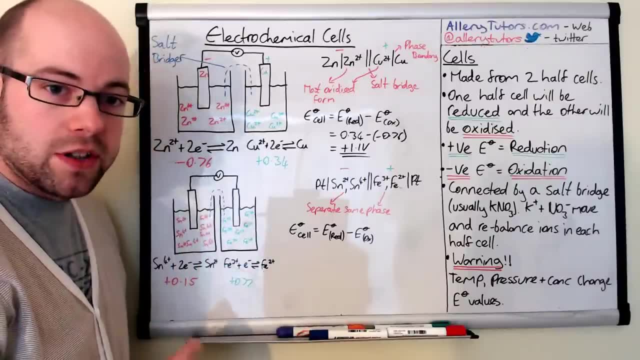 So we've got- in this case we've got tin two plus and tin four plus in a beaker, And here we've got Fe three plus and Fe two plus. Neither of these are solids, they're all aqueous, So we need an electrode to be able to carry the current, and the electrode we choose is: 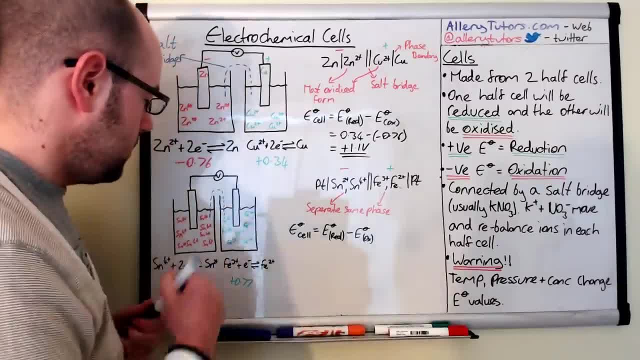 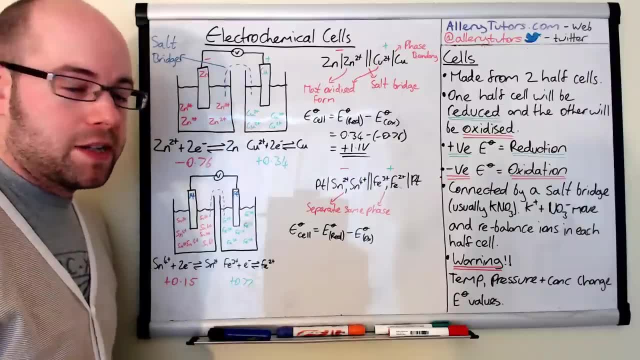 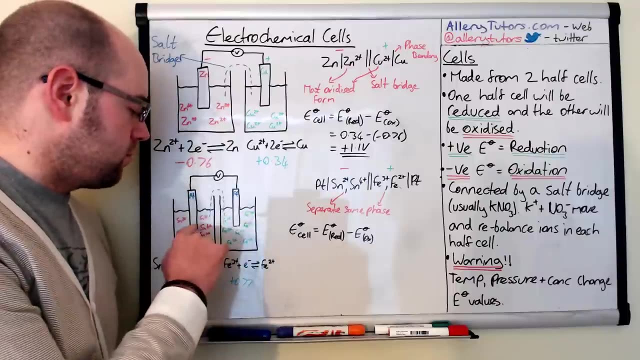 platinum electrode. So I'm just going to label that on there. So these two electrodes are platinum. put PT in there. Platinum is a really unreacted metal so it's not going to interfere with our ions And also it's a good conductive electricity so it allows us to move the electrons from. 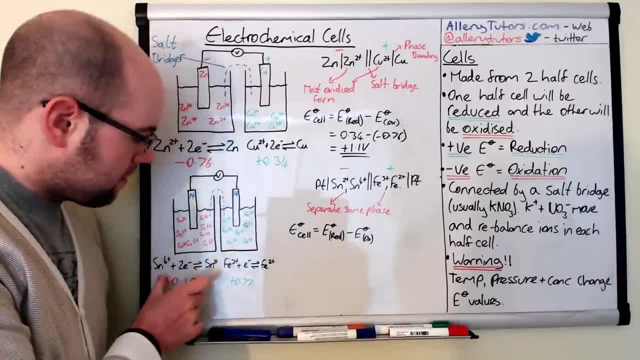 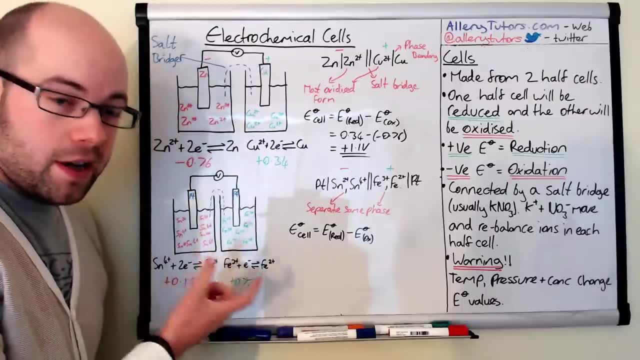 one side to the other. Now I've written down our plus 0.15 and plus 0.77.. Now the most negative out of these two is obviously the 0.15.. It's more negative than this one, even though it's got a positive value. it's smaller, it's. closer to the negative end. So, because this is effectively the most negative one, it's going to be a positive one. So I've written down the positive value. it's smaller, it's closer to the negative end. So, because this is effectively the most negative one, it's going to be a positive one. 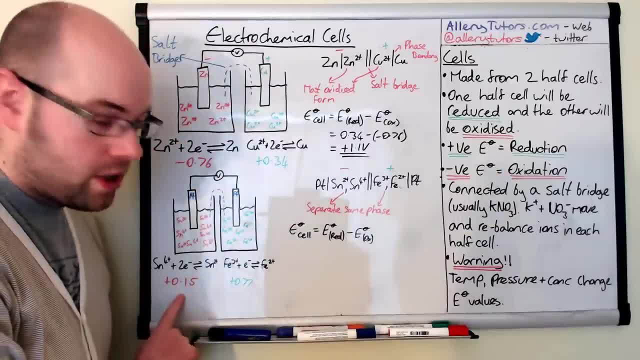 So because this is effectively the most negative one, it's going to be a positive one. So because this is effectively the most negative one, it's going to be a positive one. That means we've got just a very small tip first, which simplyvey above the 0.15 Beetle. 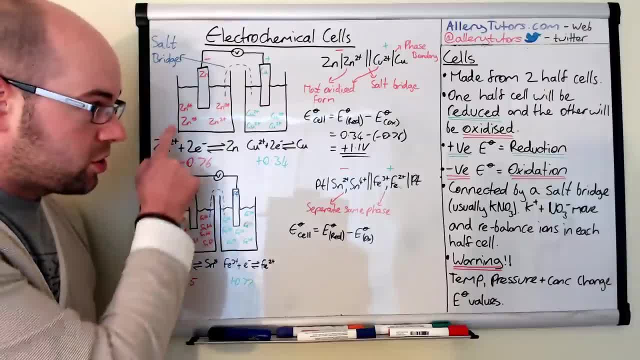 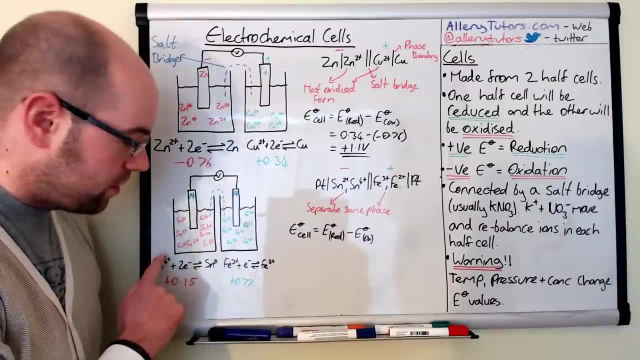 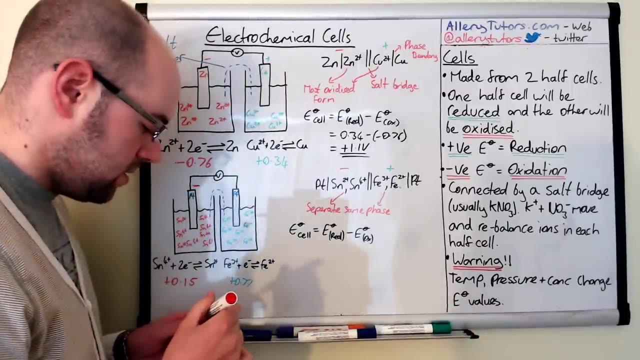 there's a little bit of crosses here in theify: arent baj 아이�赣. That means we've got a very small tip bit between 0.15 Beetle and 0.Ф and also another of the ones you need to give me this time, which is this little bit here. 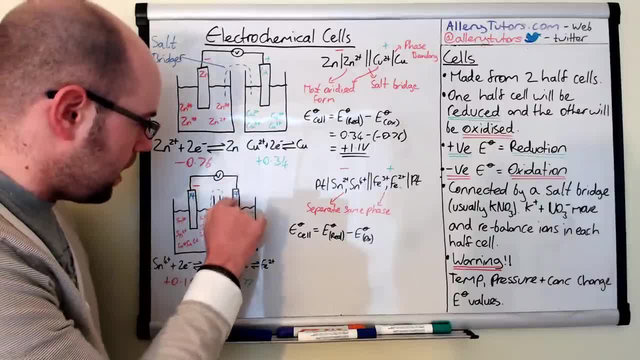 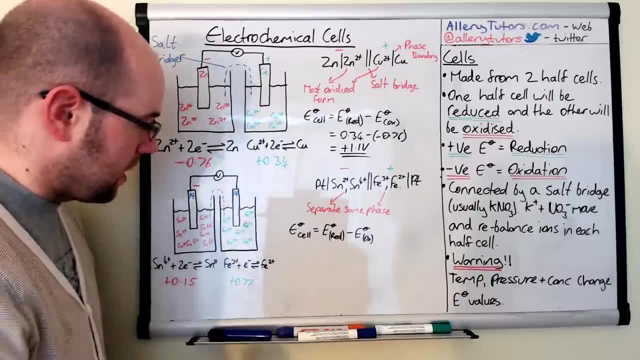 I'ts just a little bit wider than 0.15 Beetle and 0.32ät'前赣s, then 0.29 Battle Hat. Fe3 plus will pick up the electrons to form Fe2 plus, and that's what's happening here. 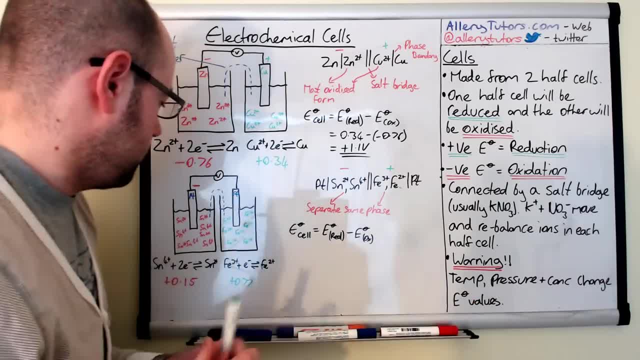 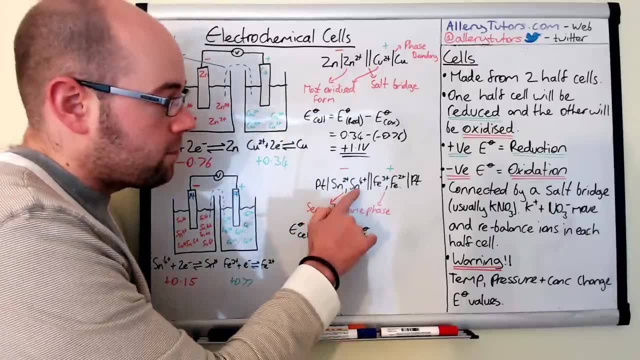 So we say that that is positive. So we're going to put that in there, that's positive. Okay, again, I've written our cell representation here Again. remember the most oxidized form? well, the negative electrode is written on the left-hand side. 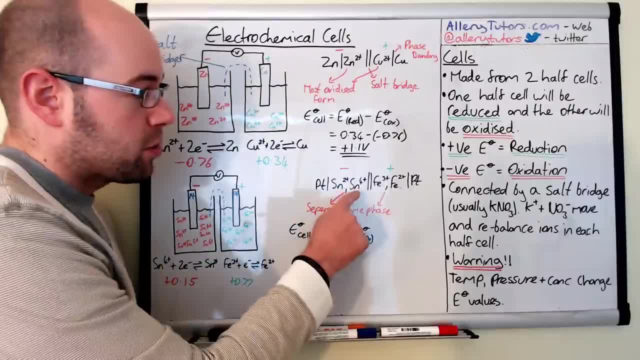 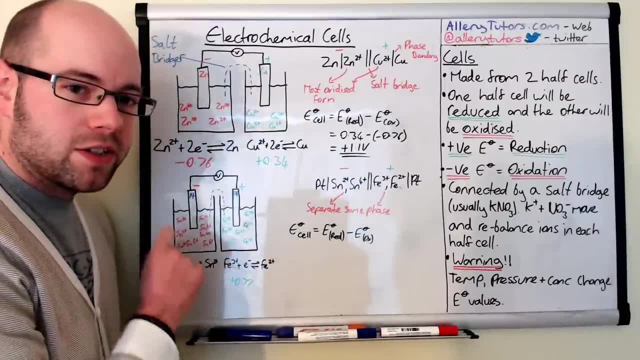 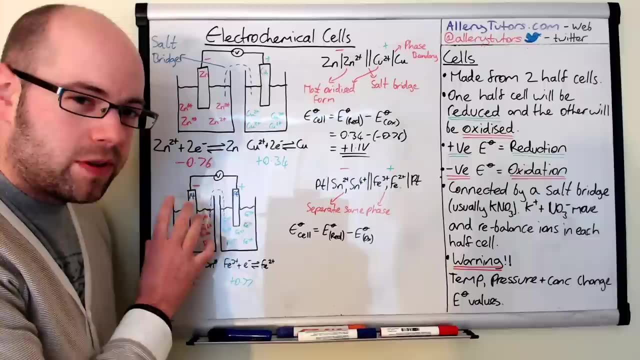 and the positive electrode is written on the right-hand side. The most oxidized form is written closest to the salt bridge. Now this is a little bit different because we don't actually have a solid metal electrode. We've actually got- well, we've got- a platinum electrode here, but we've got two ions and both of these are in solution. 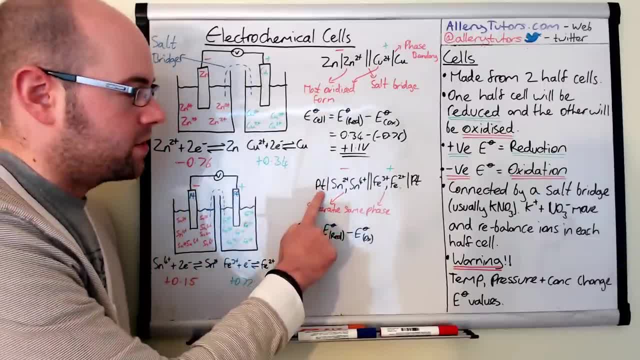 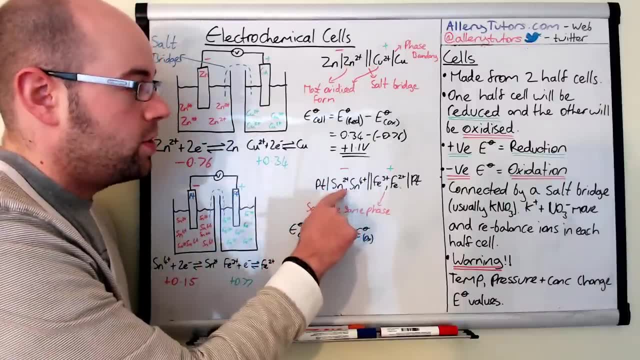 So what we have to do is write it like this: We put platinum there on the left-hand side, The solid line represents the phase boundary between solid and solution, And then we have two ions that are in solution Now. the most oxidized form of them two ions is Tin4+. 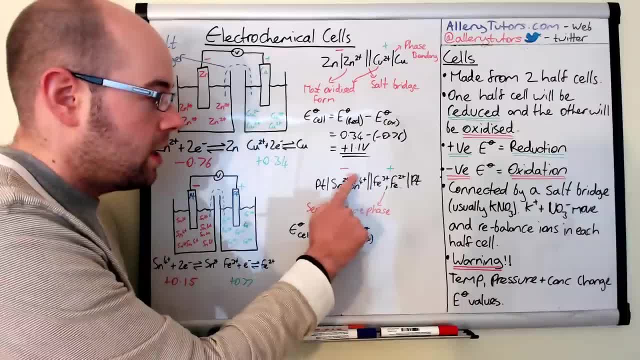 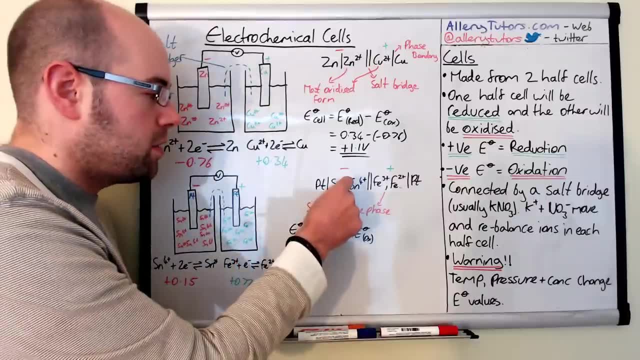 This goes on the right-hand side, closest to the salt bridge, and the Tin2 plus goes a little bit Now because these are both in solution. there's no phase boundary here, So what we do is we separate it with a comma because they're in the same phase. 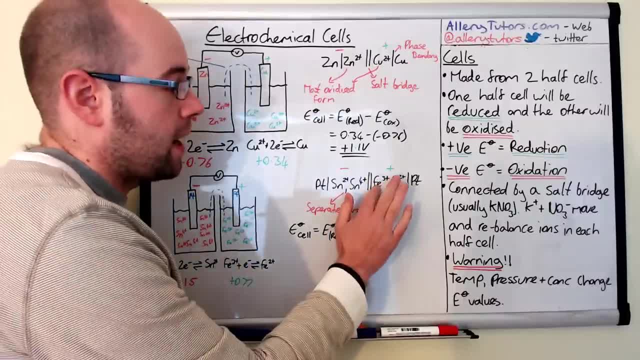 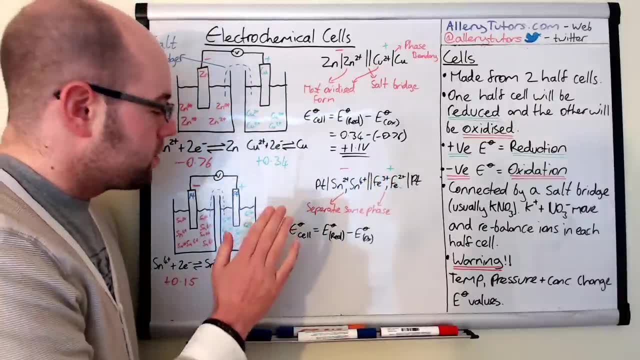 They're both aqueous, and on the right-hand side we've got iron3 plus, iron2 plus and platinum, Again most oxidized form closest to the salt bridge, which is the double ion. Okay, so we're going to work out the E-naught of the cell of this one as well. 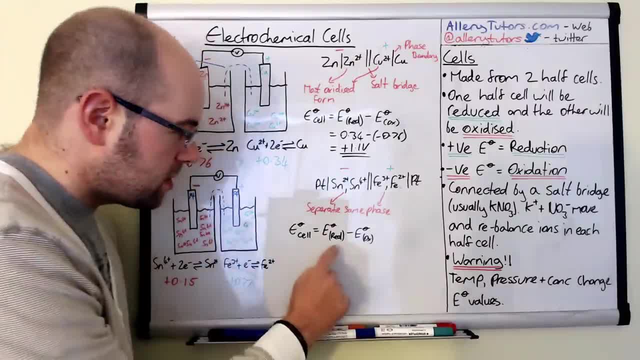 Both of these are positive values. So we're going to take E-naught of the reduced form, which is the green number there. So we're going to take E-naught of the reduced form, which is the green number there. So we're just going to put 0.77.. 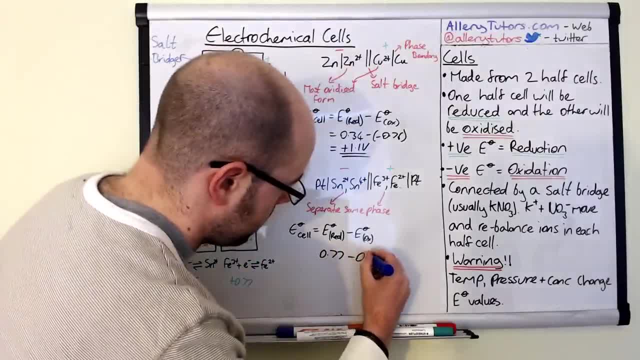 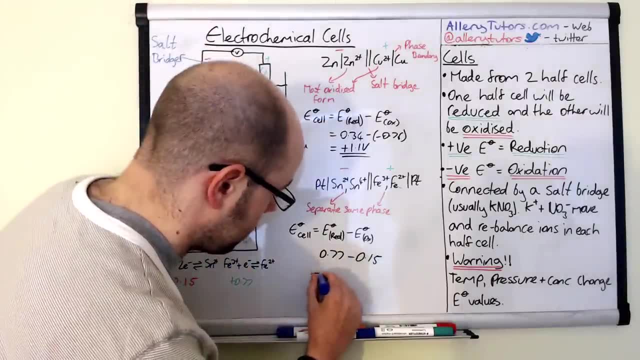 And we're going to subtract that away from 0.15, because that is the oxidized form. So this is the Tin2 plus going backwards And that is going to create an E-naught value of the cell of 0.62 volts. 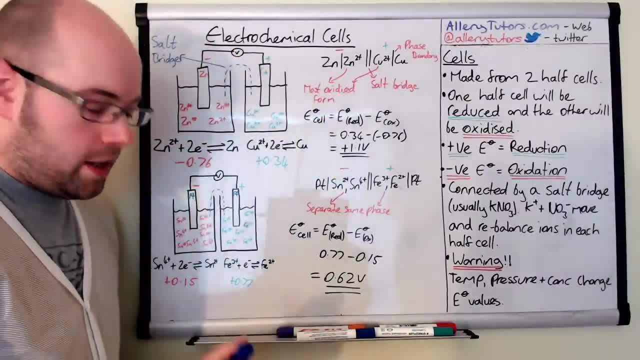 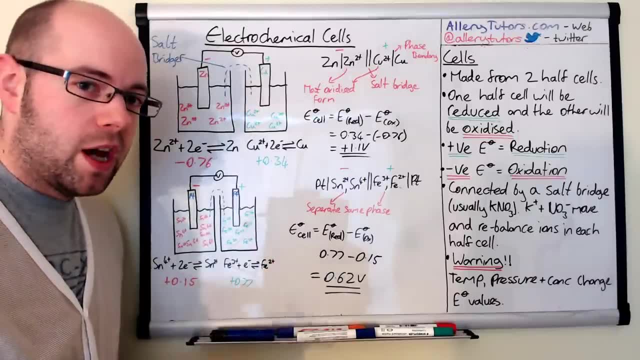 And this is the reading that we'll see on our voltmeter. Now you've got to be able to work out E-naughts of cells, of full cells, by using these equations. That's really important. You've got to understand that one of them is negative and one of them is positive. 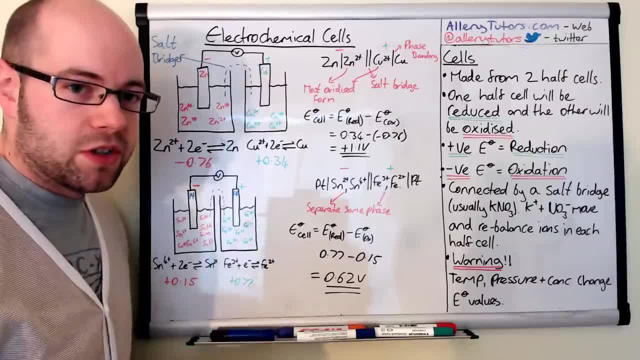 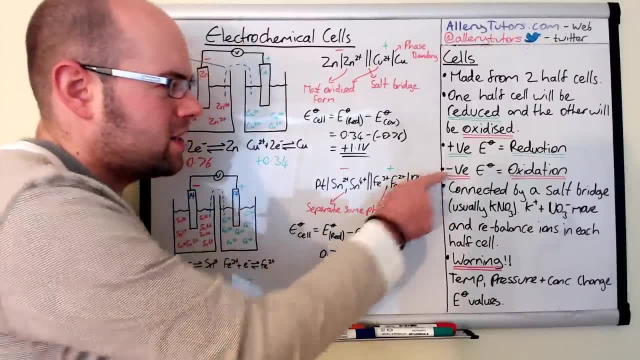 And the one that is negative is always the reaction that's undergoing oxidation And that number is always going to be the most negative number. So you can kind of remind yourself: The most negative E-naught value is the negative electrode, And that's where the electrons are being produced. 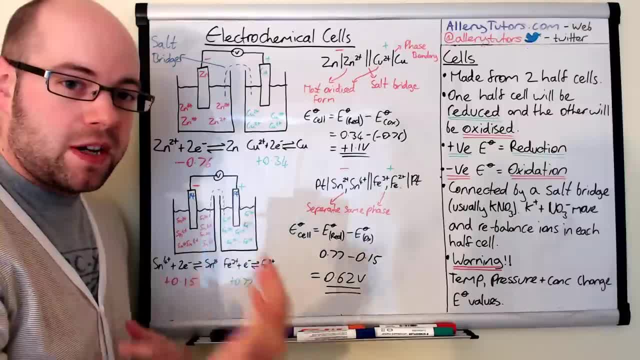 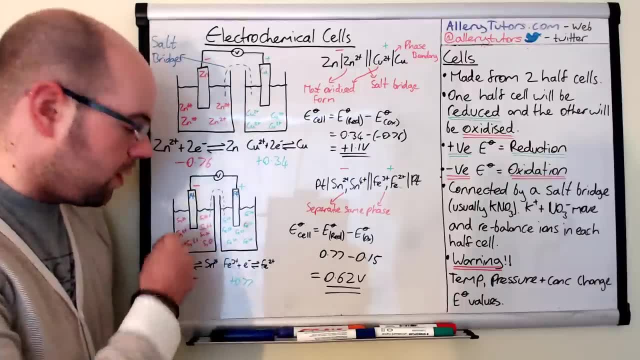 And remember always in electrode potentials. when you see them on a data sheet, they're always written in the reduced form. So if your cell is being oxidized, you have to swap the reaction around or the equation around and you go backwards instead. 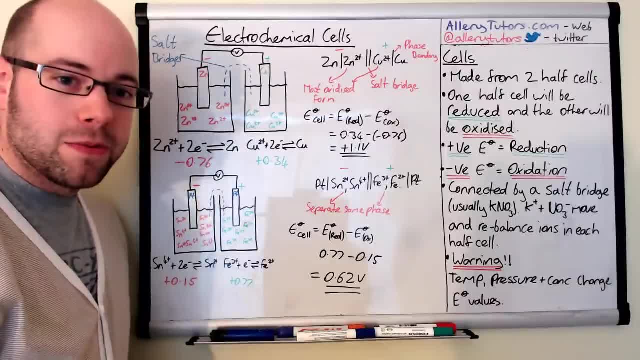 because this is the reversible reaction. But that's it. Hope that helps. Bye. 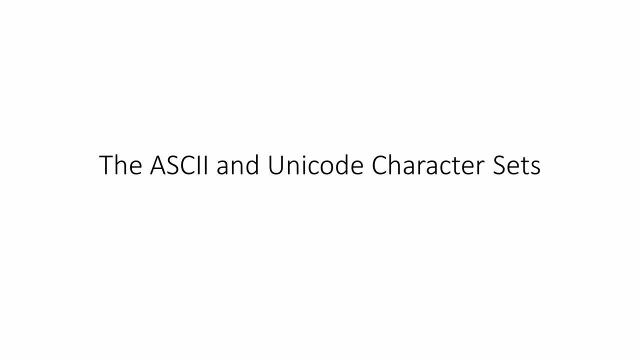 Put simply, a character set is the list of characters that your computer can understand, But there is of course more to it than that. All computer scientists, and particularly programmers, should understand the fundamental principles of character sets, character encodings and Unicode. Only then can they develop computer systems that will work with text in any language. 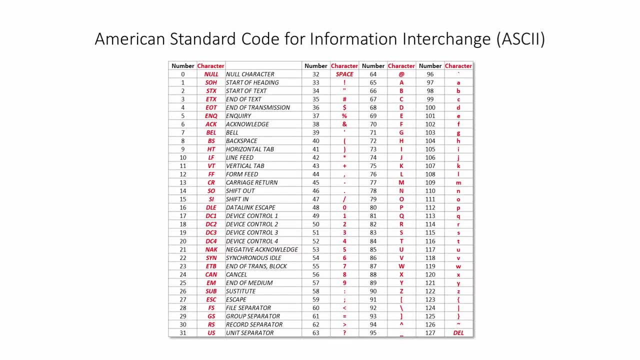 Once upon a time, the only characters that computer scientists cared much about were English letters, digits 0 to 9, and a handful of punctuation symbols. There was a system for representing these characters called ASCII, the American Standard Code for Information Interchange. ASCII could represent every character on a standard keyboard and a few unprintable. 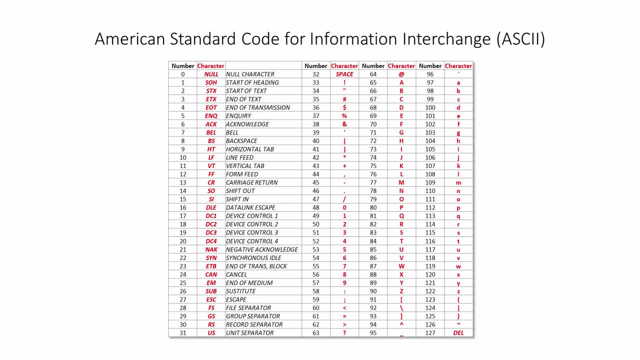 control characters using a number between 0 and 127.. Characters 0 to 31 represented unprintable control characters. For example: 7, bell made your computer beep. Number 12, form feed caused your printer to eject to the current.